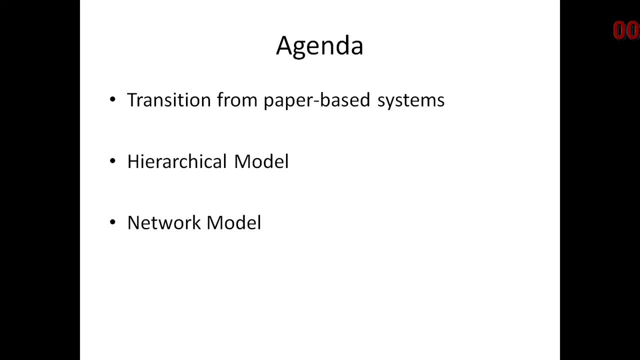 They do. but many large companies, large retail companies, converted to computerized systems using the hierarchical model beginning in the early 1960s. We're going to see the thought process that people used to design these systems. Hint, it was based on the way things were done at the time, which was paper-based. 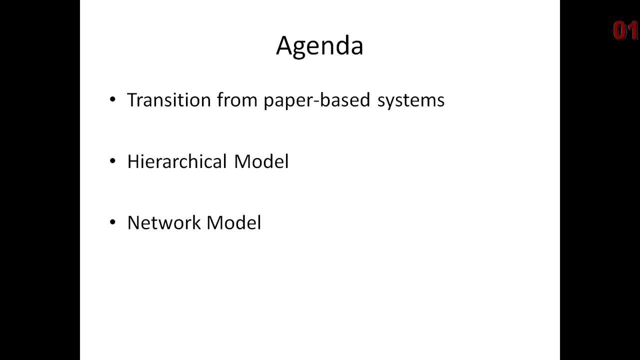 And what some of the problems were. that people ran into, what the frustrations were, what the disadvantages were to the system and how that eventually led us to what we currently use, which is a relational data model- And I'm throwing in a little bit of background. 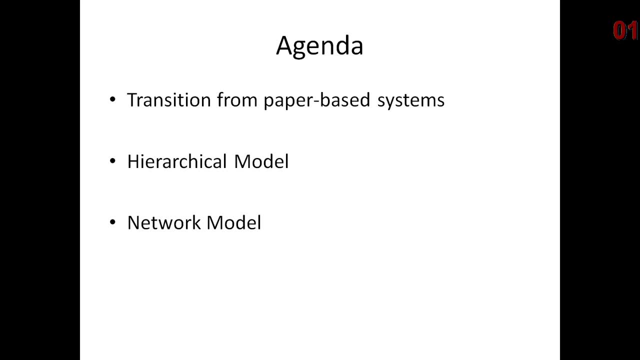 Let's talk about the network model, because that was a reaction to the problems we encountered with the hierarchical model. It didn't save much heartache, It was still problematic and was not much of an improvement over the hierarchical model, But it's important that we are aware of these because of the approach people took. 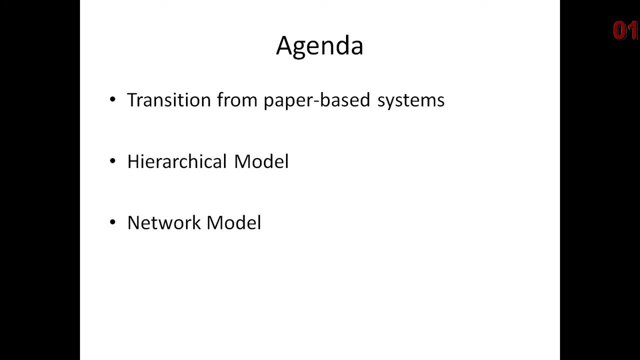 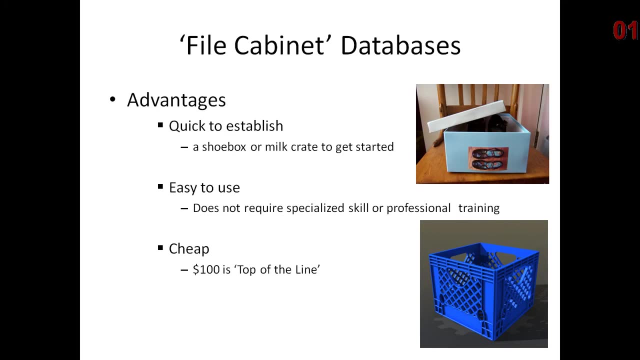 And we want to avoid those same design flaws. So, as a reminder, we've seen this already in our previous module on file cabinet or paper-based database systems. There were advantages to the paper-based system. This is how business was done for centuries, up until 1950s. 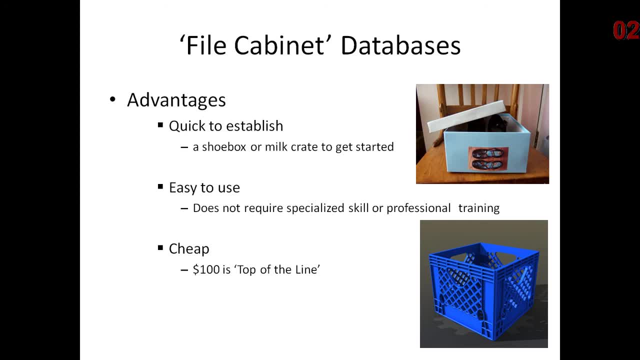 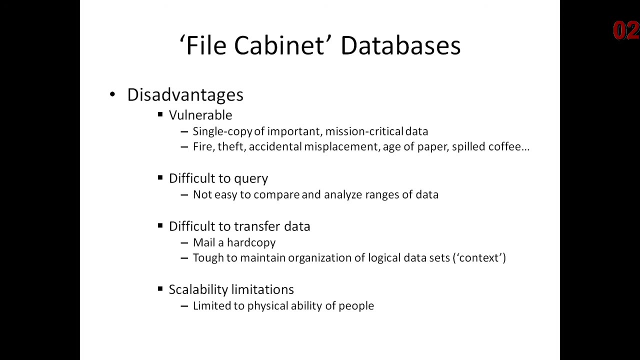 Obviously quick to establish, easy to use, cheap. It follows a relatively simple way of organizing items. Problems: Problems, as we've seen: Vulnerable. It's not very secure, Difficult to query, Very intensive. Imagine having to account for all the books in a library, physical books in a library, without going through the card catalog. 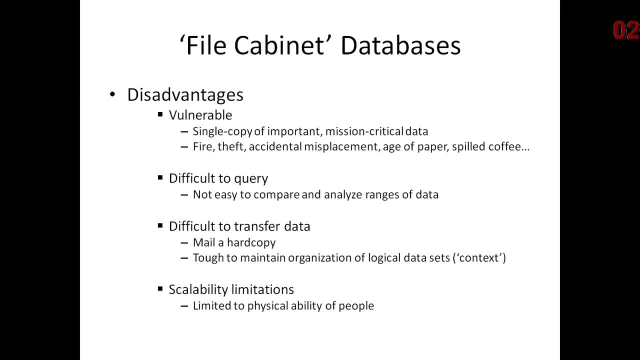 Those of us that are old enough remember the card catalogs. Nowadays, in an undergraduate course you say, hey the card catalog, And blank stares. Nobody knows what a card catalog is. Then obviously the paper-based system is difficult to transfer data, making even photocopies. 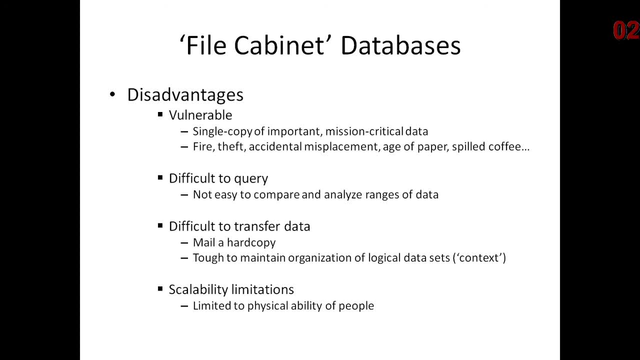 We begin to water down our integrity. We lose control of the many copies of records. Problematic- And then, obviously, scalability limitations. We're limited to the ability of people to physically manage and process paper File cabinet database systems. again, that's how business was done for centuries. 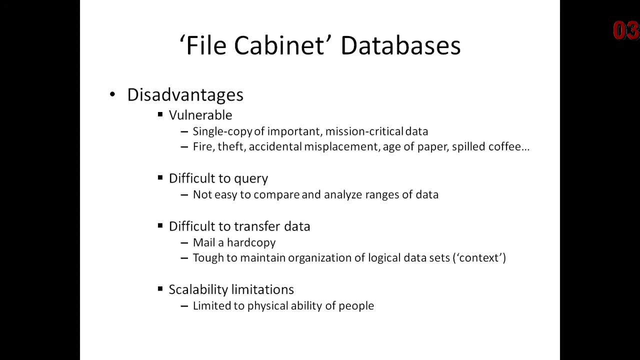 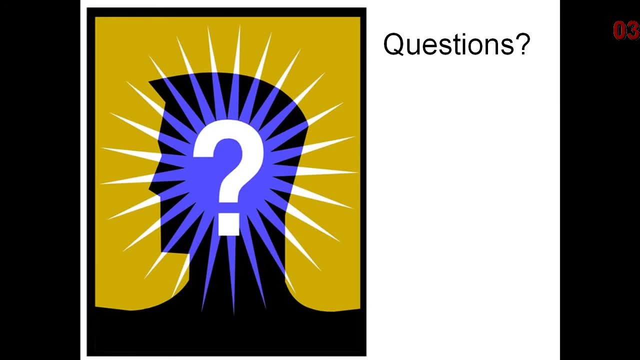 It worked. It affected how our economy was regional or local, And we'll talk about that, perhaps. But we have evolved. And how did we evolve? Again, I put a question slide in here. Feel free to send questions to me. gthay at uwedu. 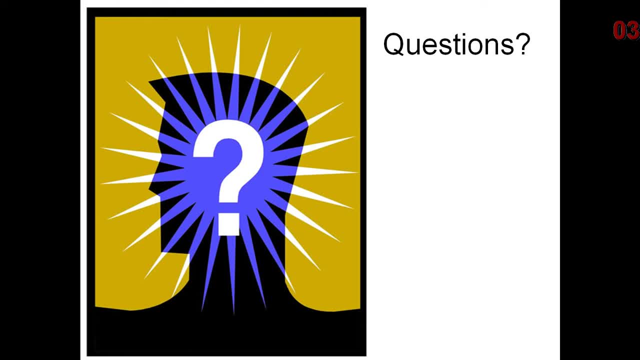 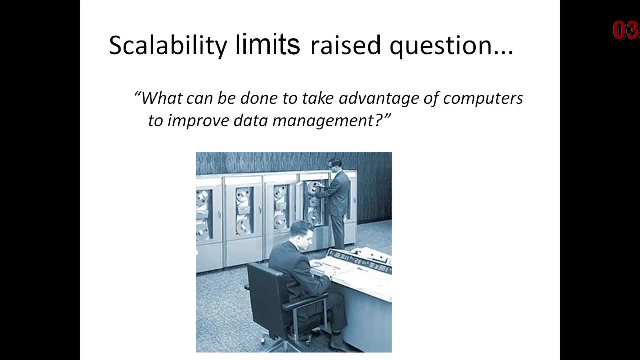 I love questions because that helps me stay abreast with where students are and what we're learning. So again, we had scalability limitations with paper-based systems. Large companies- Think of Sears, perhaps IBM- obviously Companies that did large numbers of transactions. 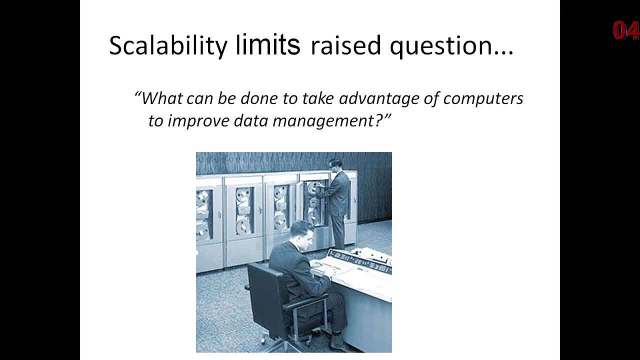 JCPenney. I'm thinking of retail companies because they probably did more volume of transactions than other companies. What can be done to take advantage of computers to improve data management? Now, this picture shows actually a mainframe computer, probably 1960.. 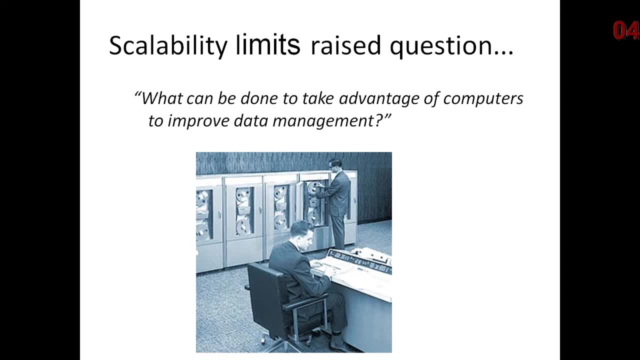 And you see the reel-to-reel tapes there You see people manually handling tape- Not very efficient. I'm probably going to guess that there's more storage space on a very cheap cell phone than would take up an entire room in 1960.. 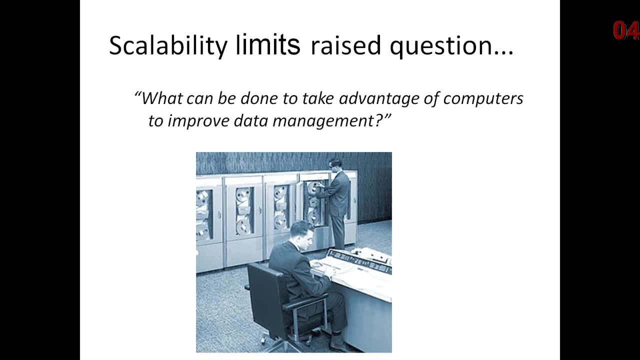 Literally Megabytes take up an entire floor in an office building in 1960. Megabytes: On a cheap phone you probably have at least 4 gigabytes. If you're spending more than $150 on a phone, you probably have 32 gigabytes of storage space. 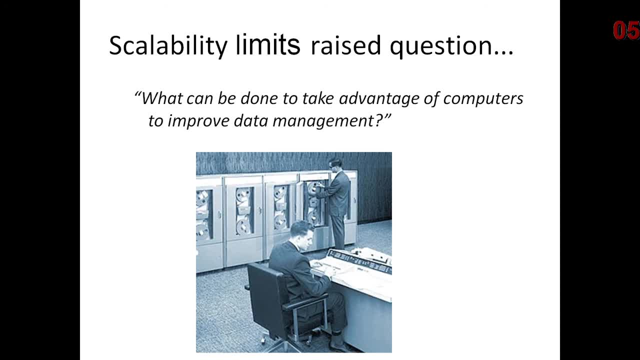 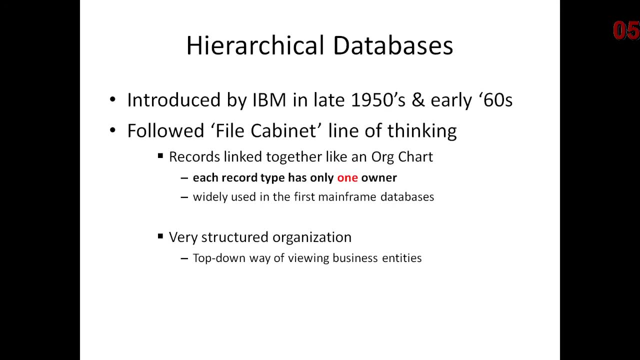 Which would take up a whole building. perhaps We'll talk about the way hardware has evolved as well in a different model. So let's get a little bit deeper into hierarchical database designs And the reason we're doing this. again, there were problems. 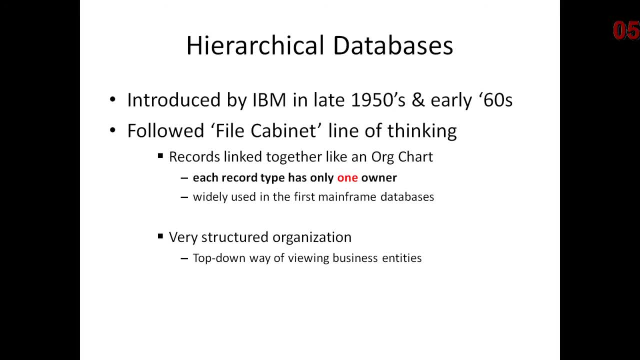 The problems were that engineers approached the design structure of computerized databases in the same form that we were used to organizing paper, And it made sense. That's how we've been organizing data for centuries. Why make any changes? It worked. It may have been cumbersome, but obviously the thought was: with computers it should go better. 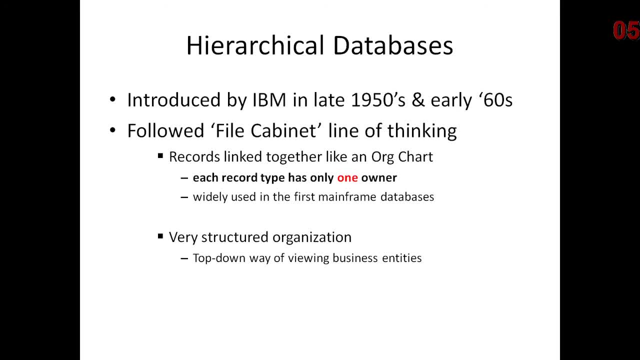 It should go faster, And we'll see that it really, truly didn't So. hierarchical data model introduced by IBM late 1950s, It followed the file cabinet or paper-based line of thinking And records had, as the name suggests, a hierarchy. 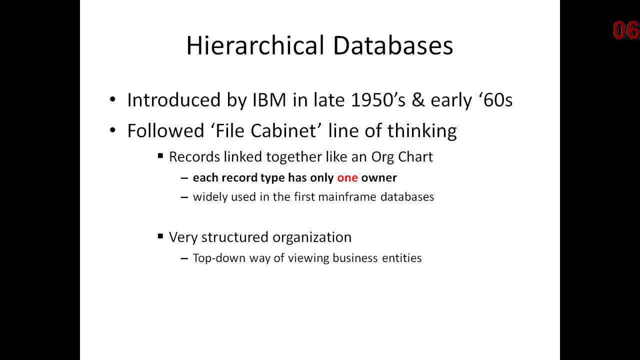 So there was one folder, one drawer, And that translated to one database, one file where records were stored. It was a top-down approach, So each record- I put this in bold- each record type has only one owner. There is one way in to locate a record, a transaction. 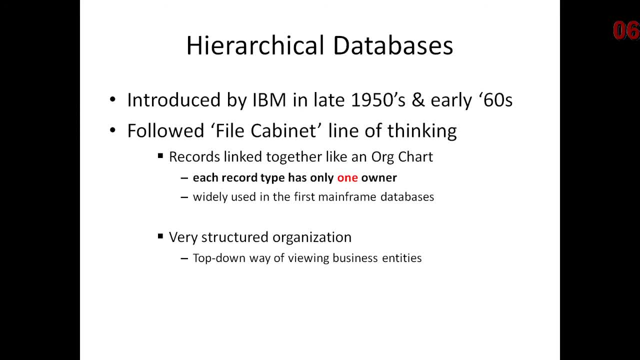 And, for example, it could be at a store level. So Let's say JCPenney has a point of sale. They are tracking all transactions, all items sold. They may have a hundred stores To do a roll-up of all transactions for a particular day across the entire company. 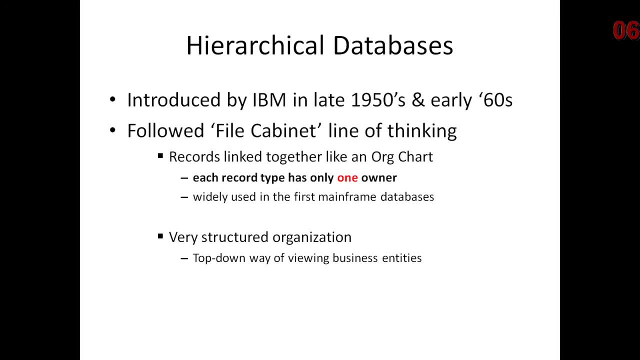 they could not summarize across stores. Each store had to be investigated and summarized individually. It may seem like, yeah, so Well, that's not how we kind of do it. in today's world of database design, It's possible that there might be some scenarios where we are rolling up on each individual store level. 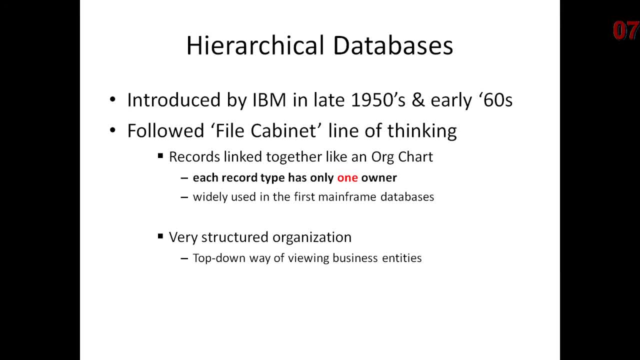 But the idea should be that we're able to roll up across all stores at the same time. We will see an example here shortly. The idea is it's not very efficient If we have to dive down vertically into each file. and let's say there's a hundred files, one for each store. 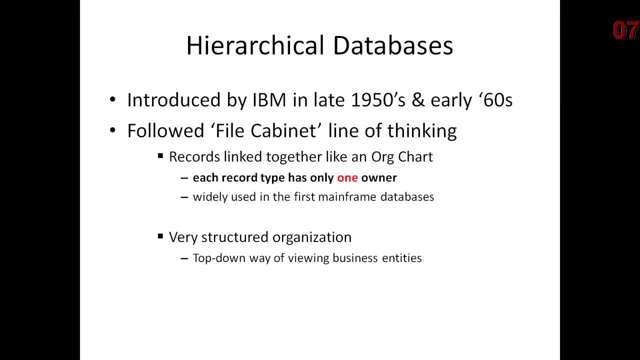 we're diving down in sequence in each file to run the same query a hundred times. It doesn't quite. It doesn't scale very well. This was a very structured organization, top-down way of viewing business entities. This is somewhat of a model. 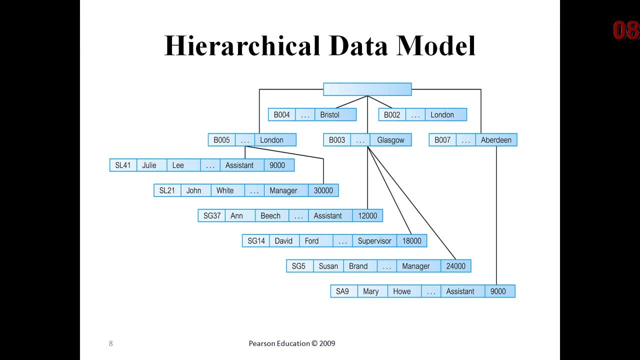 This is borrowed from the book Hierarchical Data Model. So this represents a bank and different branches, And each branch has employees And to determine if an employee where an employee works, for example, we would have to dive vertically into each file, into each branch. 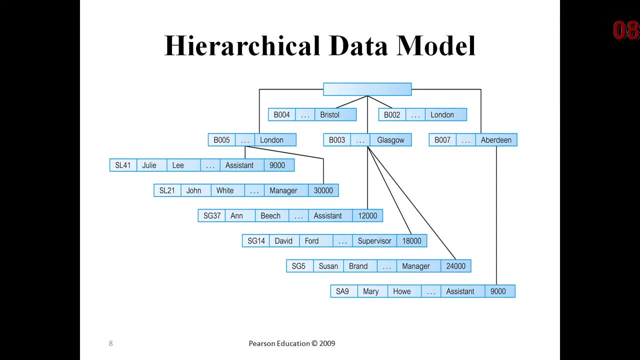 Does John White work for the branch in London? Let's look. No, All right. Well, in this case he does. But let's say we started with Aberdeen. Does John White work for the branch in Aberdeen? And you do a scan? 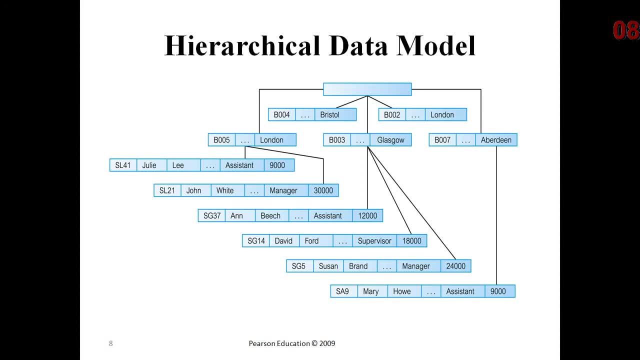 Nope. Well, let's see if John White works in Glasgow- Nope, You do a scan. Imagine having 300 branches. Not very efficient looking for an employee. It is much better nowadays where we just type in White, do a search under employee. 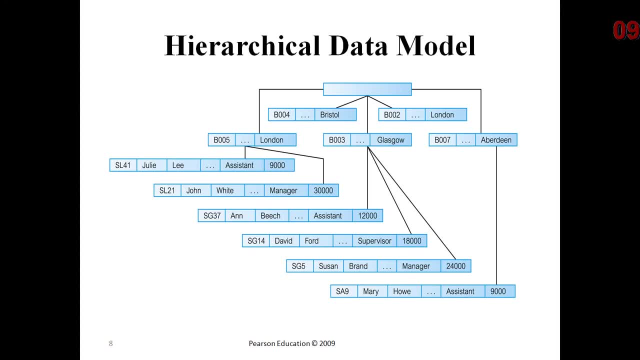 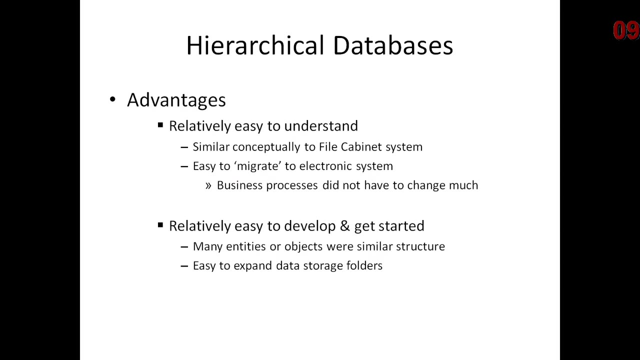 and try and see what comes up. Oh, the person works for London branch. A lot easier than having to vertically dive into each potential location. There were some advantages with the hierarchical database design, Since businesses were organized in a paper-based system already. 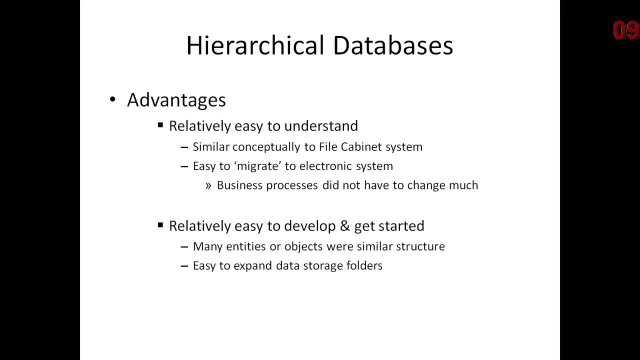 it wasn't that difficult to incorporate computers Very, very similar conceptually to the file cabinet system. This was an advantage If there was a team of 30 paper processors- order processing people. pretty much they kept their job. They knew how to process paper. 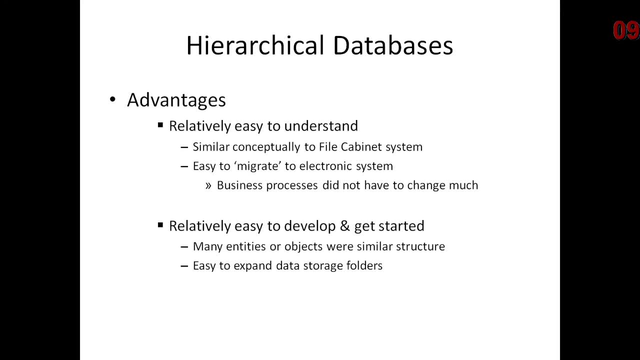 They knew how to process paper on a computer. That's how the forms were built. It was easy to migrate to an electronic system. They didn't have to change much Now. well, we'll get to the disadvantages in a brief second. 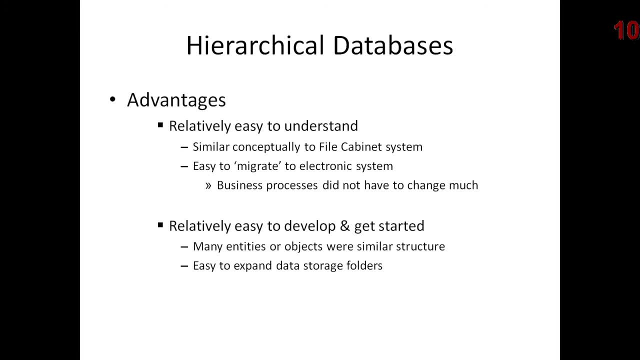 Relatively easy to develop and get started. Many entities or objects were similar in structure and easy to expand. data storage folders, Meaning the way that the business was doing business- the way an organization or company was doing business- didn't have to change much. 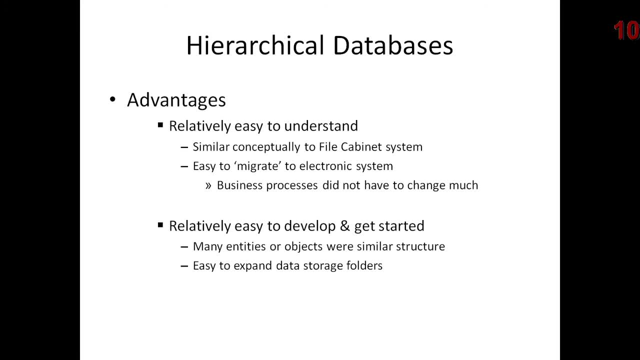 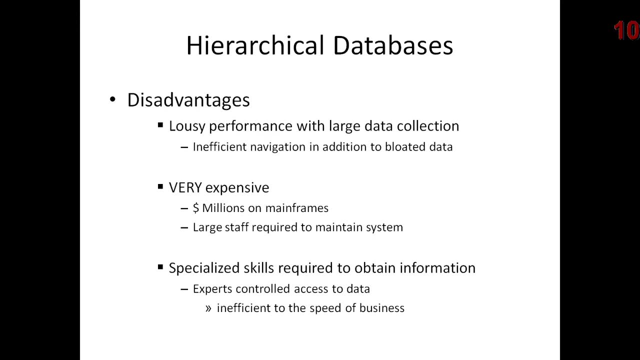 The system as designed followed existing business practices Disadvantages: Well, we had lousy performance with large data collection. It was not able to be determined with a paper, manual-based system where the bottlenecks were. It was just people. Add more people and we would be able to. 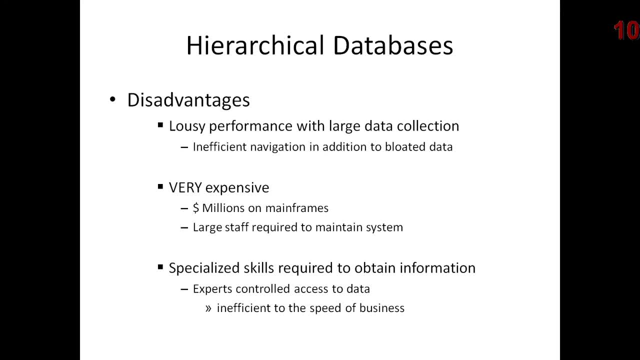 process, more paper. Well, once we got onto the computer that process went faster. It did go faster But we determined we were able to see that at some point it would bog down. And it didn't matter how many, how much bigger the computer was. 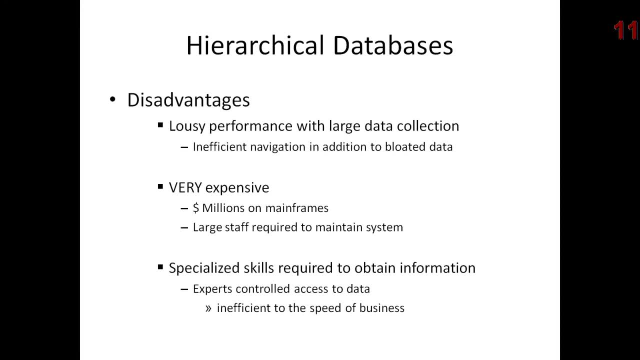 It had to do with referencing data and objects and people trying to get into the same files at the same time And we couldn't make the computers big enough And it would slow down. An example would be orders for the last week. Well, if that is generating. 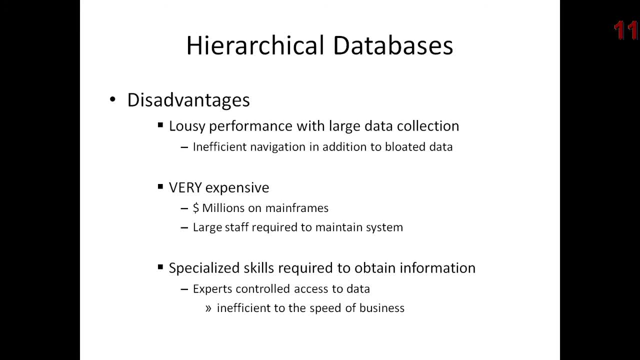 let's say, 80% of the read activity in a large company. 80% of the queries are dealing with data from the last 7 to 10 days. We're going to be all. it's like having one box of pizza. 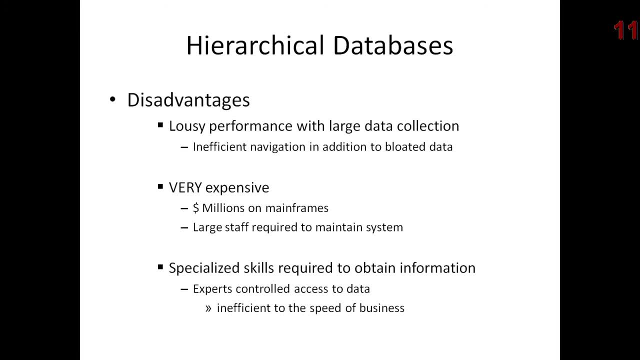 and everyone trying to go for one box of pizza. I know this because I've bought pizza for a bunch of junior high school kids before And it's like wow, that's a mess. So I use that as an example. Lousy performance at a certain point. 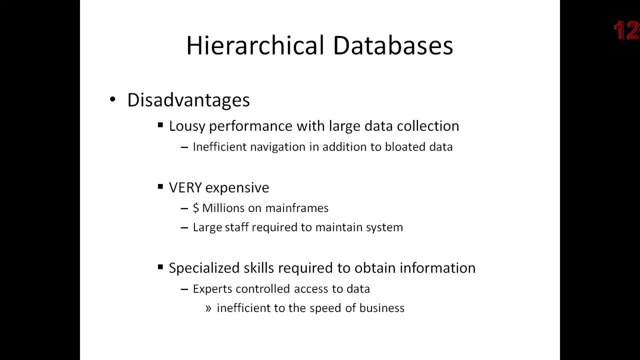 We hit that relatively early with hierarchical database systems, Inefficient navigation, in addition to bloated data. So the bloated data is going to be key Because once we hit the bottleneck, once it started slowing down, people started making secret copies of data. 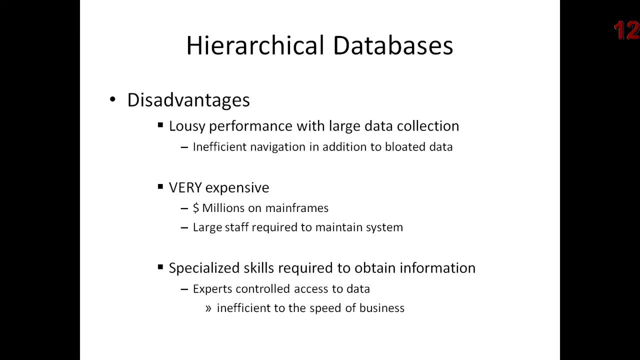 New files that kept their data. Let's say I'm a sales rep or a person that deals, a customer rep that deals with a finite list of organizations- stores, suppliers, customers, whatever it might be- And if I share that with everybody else in the company? 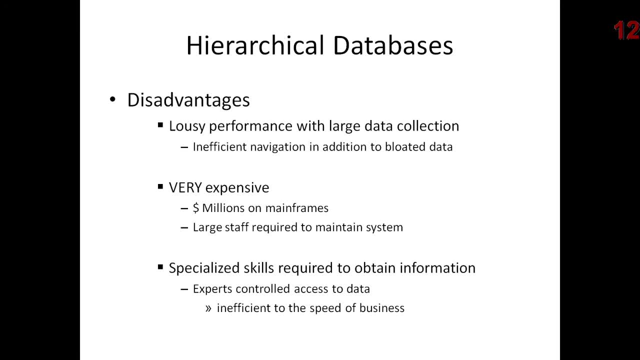 I get stuck in the freeway trying to get to the data Metaphor. I get stuck trying to get to the data And it's frustrating. So I say: tell you what. I'm just going to keep my data local. I'm going to make a new file. 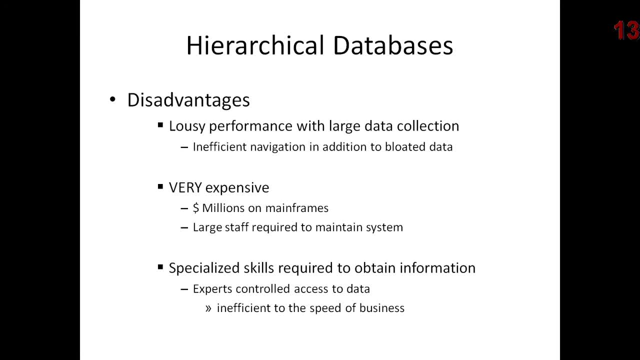 I'm going to get sneaky. That's just human nature. We get frustrated. We try and find a way around the bottleneck. Well, use, extend that a little bit. What happens if we have sneaky data? Well, it doesn't always get broadcast. 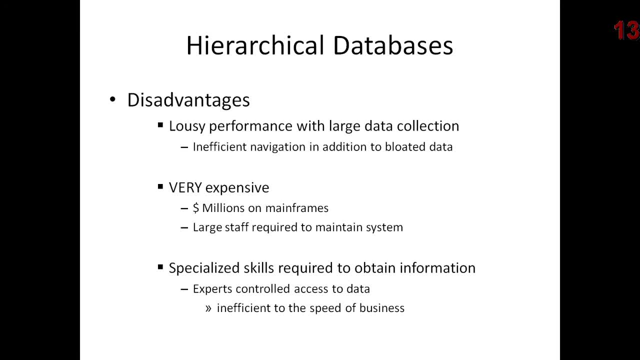 that it is the real data. So old data, inefficient, updated data is being used by everybody else in the company. So if they want to contact XYZ- company that I own and I'm maintaining- but I'm not sharing my local data because I don't want everyone else to come in- 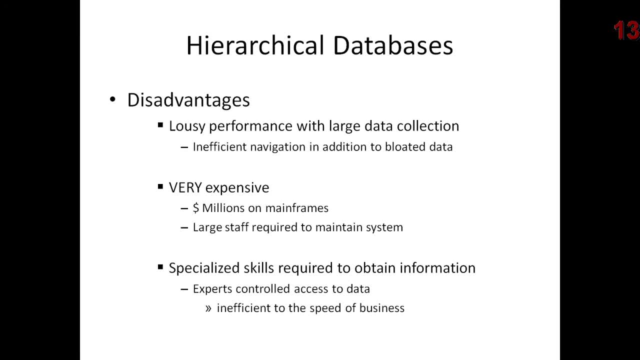 and deal with it. This is hiding that extra box of pizza. It might be the cheese cheesy bread. So what happened to the cheesy bread? I don't know, Greg, what do you got underneath the pillow over there? I got the cheesy bread. 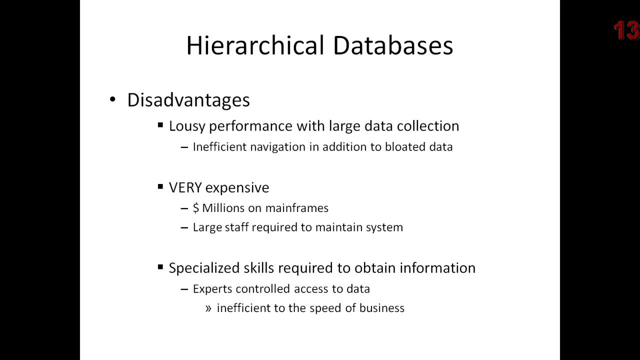 Okay, So this is an example of having the extra data somewhere else in the system. Now, that didn't always happen, but it happened often enough that it became an issue. Also, it was inefficient to navigate vertically, like I was showing with the different branches. 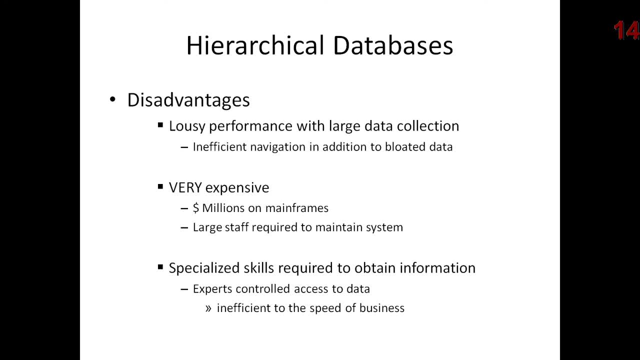 trying to find one single employee, We would have many needless queries. I say needless nowadays, because of how systems are designed, We can answer those questions very quickly. However, when we don't know where the particular supplier or employee or customer, which file they live in, 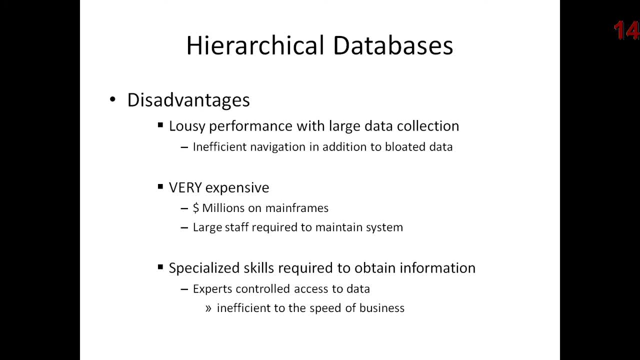 we'd have to run a random set of queries across many, many, many files, And so a lot of that activity are just search missions, hunt and search missions- And it was not very efficient, So we would have to keep extra copies of data. 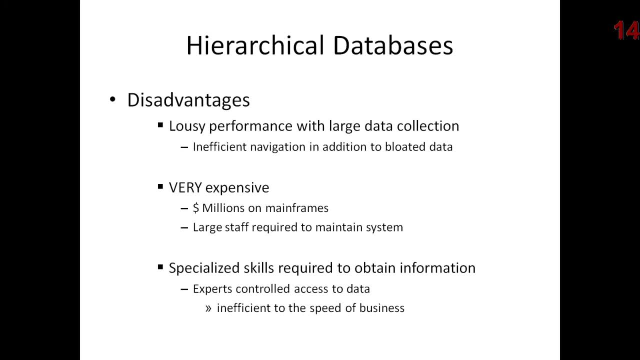 So we would have a set of records on employees. We'd have a set of records on branches. Imagine having the branch information with employees so we don't have to navigate and try and relate. okay, this is the employee that works for London. 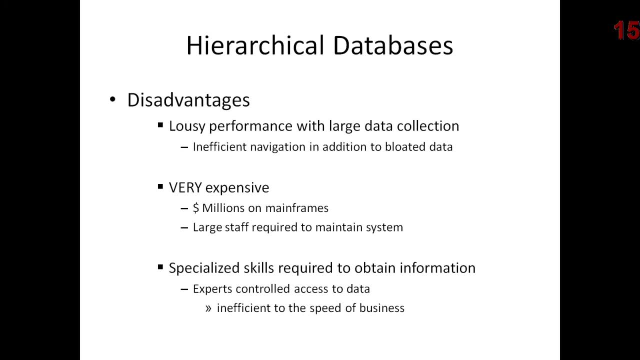 I have all of the London branch information with that employee. Then if I'm searching under branch information I'm also going to pack or stuff employee data. So I have employee data in multiple locations. I have it with the employee data centric file. 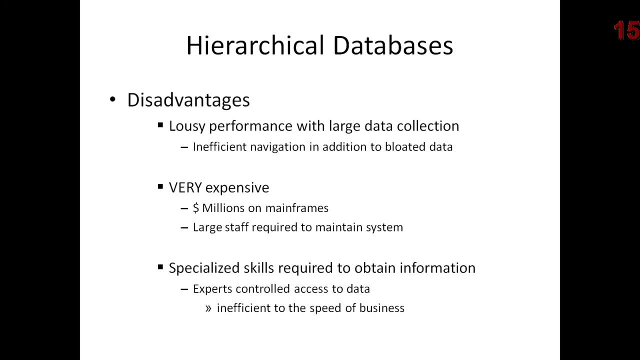 I also have it with the branch centric file: Multiple copies of the same data. okay, We're storing data on disk as if it's a paper-based system. That's how it would work in a paper-based system is that we would just have all of the information we need. 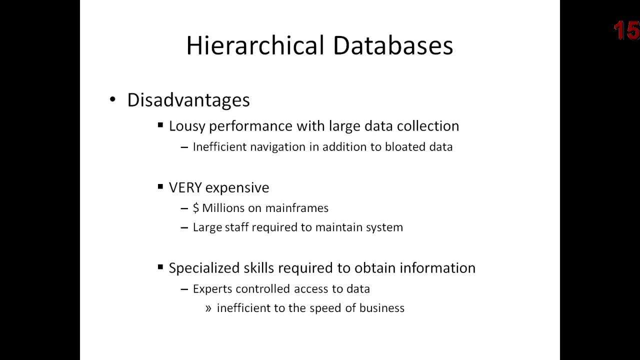 We'd store it in the form of a report because we didn't know any other way to do it. So we get bloated. We have multiple copies of the same data: Employee data, supplier data, any possible way that we're going to look at the data? 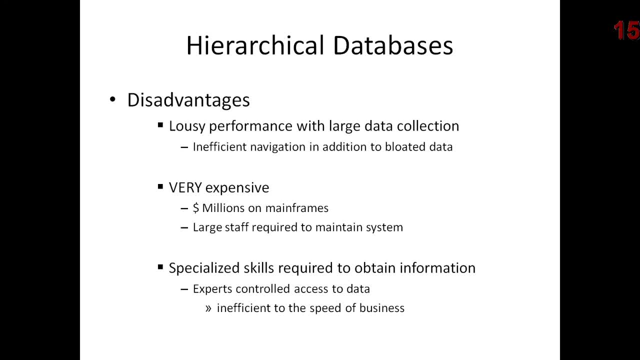 we have all of the relevant information repeated, perhaps in a different order. That's what we mean by bloated, Very expensive- I put this in caps. even That means it's like really, really expensive Millions of dollars on mainframes. 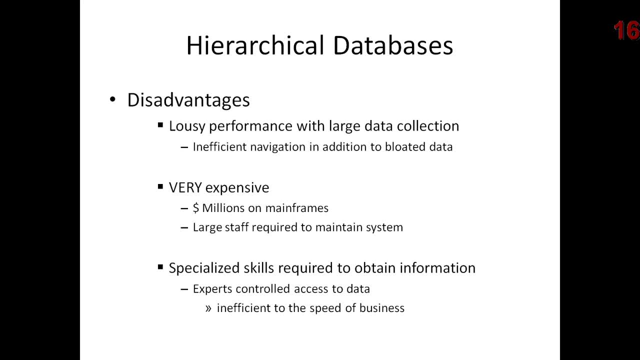 Only the very largest companies- Fortune 500,, Fortune 1000 maybe- were able to justify the expense of purchasing these large mainframes. Now remember the goal was a competitive advantage If Sears could process an order for Tuffskins from Greg Hay's mom in two weeks. versus three weeks for JCPenney. chances are. you know, we're human nature, we want to get things quicker. Okay, and maybe possibly they have less employees because they've been able to automate certain steps, So they have less expenses. 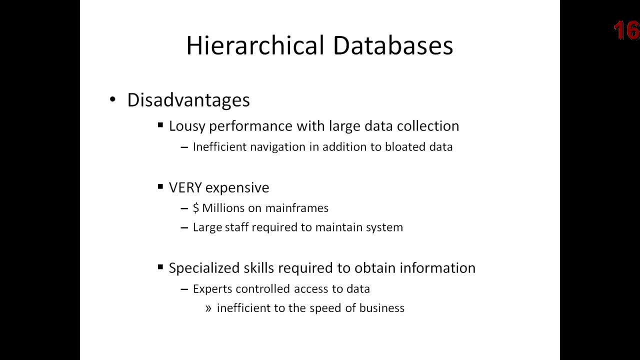 They can offer the Tuffskins cheaper. Ooh, cheaper and speedier Sounds like a winning deal And obviously it was So competitive advantage, even though there were disadvantages. people could do business faster. Organizations could go faster in processing certain aspects of their business. 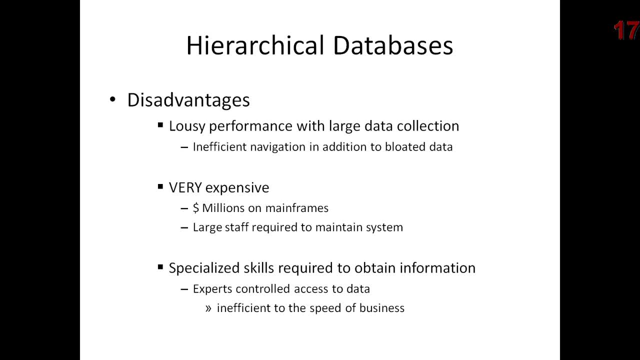 It was a winning situation, even though it cost millions of dollars. So- and I literally mean millions- Millions in 1950 would be like tens of millions now. Just do the math of inflation. okay. Large staff required to maintain system. 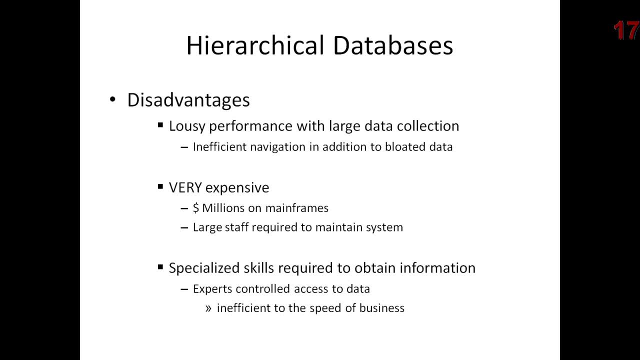 So very expensive, Entire data processing staffs- this is plural- were you know dozens of people that were highly trained, highly educated machine operators- probably mechanical engineering degrees- to manage these systems. Specialized skills required to obtain information. 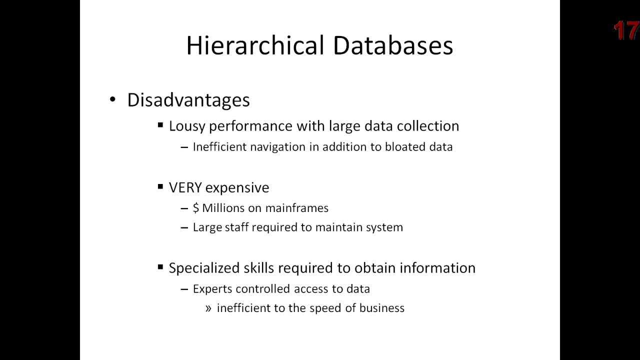 Again, same engineers managing the hardware managed the interaction. There was a data processing team, So if there was a question from a sales executive- how many widgets did we sell today? That request would be submitted to the data processing team. Please answer these questions. 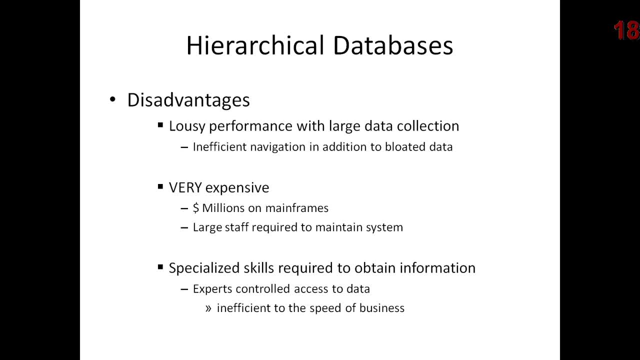 And then maybe a day later it would come back. Hey, here's the answer to your question 75. And it's like how relevant is that? When we talked about the speed of business, how fast could organizations respond to their customers? 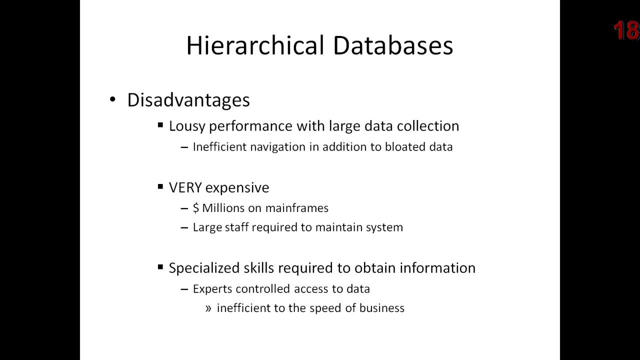 compete in a marketplace if it takes a day to get a question that we can answer, probably on a cell phone, in 15 seconds now, Imagine so. first of all, sidebar note: people get really, really frustrated if they're delayed even 20 seconds for anything nowadays. 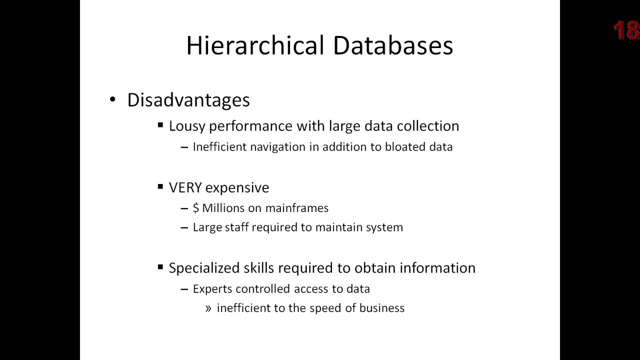 Imagine having to wait a day or two for the same question that now takes 20 seconds. Yes, people would be really, really frustrated. That said, the important part to remember about the hierarchical system is lousy performance at certain points. 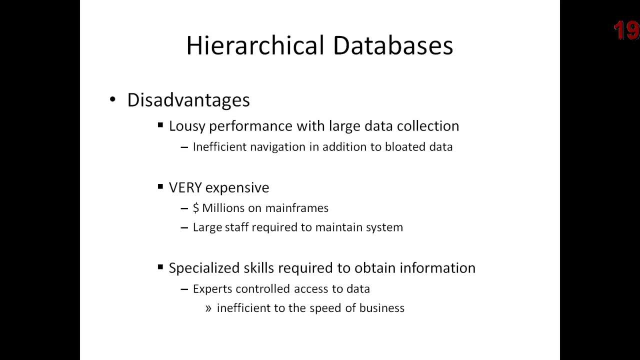 I'm going to say roughly 300, 400,000 records. Once we get beyond 300,000, 400,000 records, which is not very big, we start to see performance degradation. Now, that's just a general number. 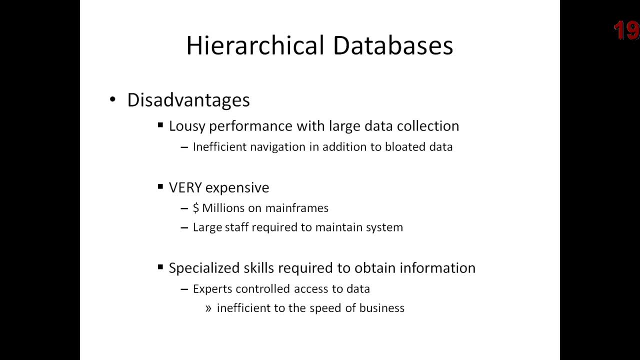 Very, very expensive, Exceptionally expensive, Only the very largest companies. You couldn't just order a laptop from Best Buy or Dell for 450 and get started with shareware database. You can't do that. You really have to invest Most. I didn't even put this down. 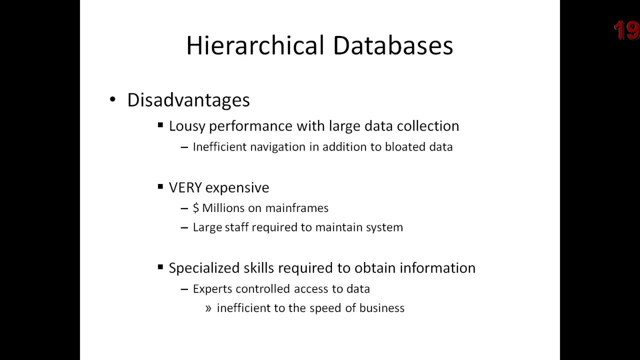 the software was often proprietary, custom built. There was no general accounting systems available. You would hire the engineers and then put them to work and say: build me an accounting system. Very, very expensive, Specialized skills required. These are the three largest takeaways. 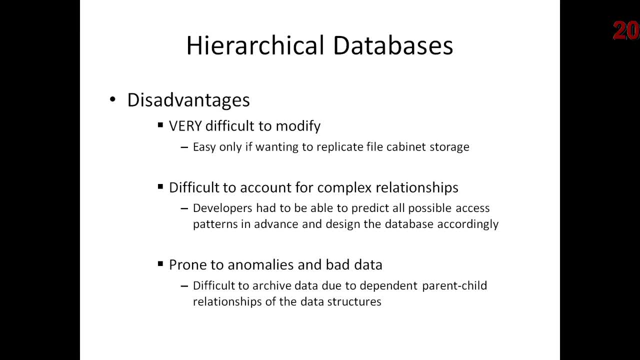 Additional takeaways for disadvantages. it was very difficult to modify The application as we like to say. so we'll learn about the N-tier architecture. This was one tier. You had a computer that you would engage with. Terminals, were we like to say. 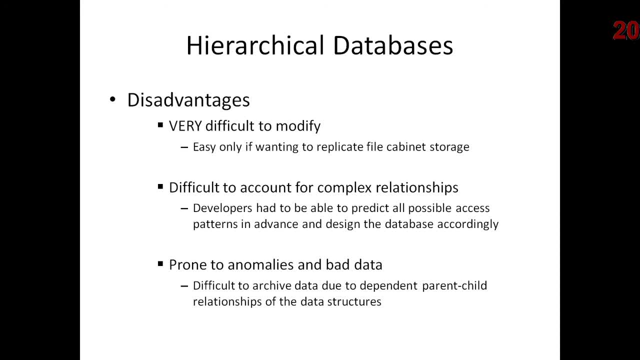 dumb terminals that were just connected to a central computer and you would interact directly on that computer. There was no client interface, as we now have. There was no middle tier, as we now have. It was very difficult to modify. The application had to know. 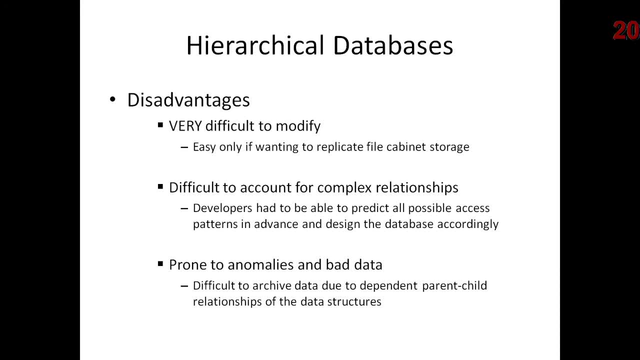 where on disk the file was located. We'll learn a little bit more about that, but that is a huge issue for making data modifications. We have a logical abstraction layer now where we reference a name, A name of a table, Where that lives physically. 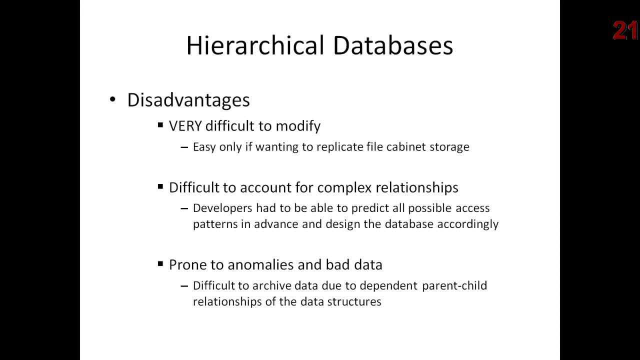 who cares Doesn't matter. That is what the database management system will manage. In the old days we had to hard code the physical file locations in the application. It's like typing in a URL in a browser, Something like that Difficult to account. 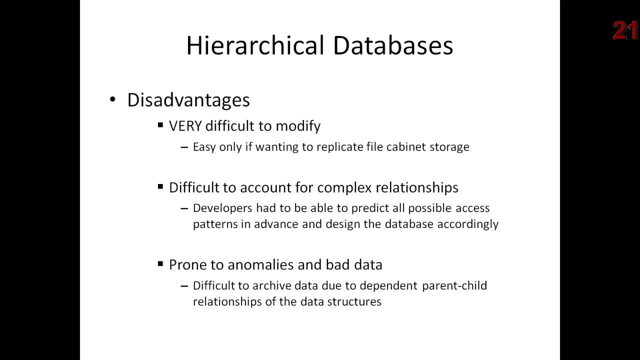 for complex relationships. Remember when I said that businesses were set up for a paper-based system? That's because that was the only way to get things done for a very long time And once so. nowadays, computers adapt to the way that businesses are organized versus. 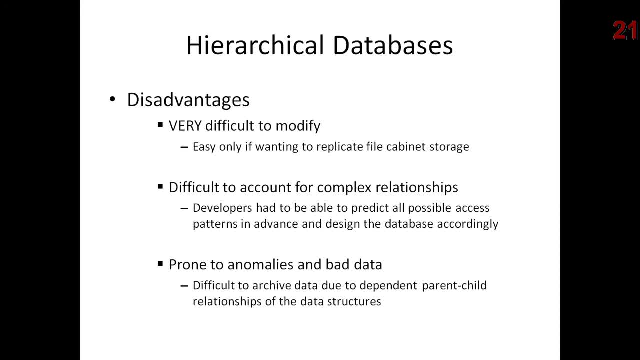 businesses adapting to the way that data was organized. There was one way, essentially, of getting data processed And businesses would staff up around the physical limitations of processing. Now that is reversed. We design the most efficient way from a people perspective and our systems react. 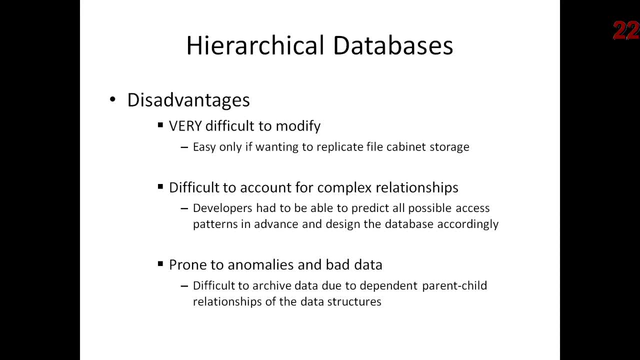 and adapt to that. So people, business operations first Build the system to support the way that the company is organized. Old days we had to account for how paper was processed And then we'd build up a staff around that. So very difficult to account. 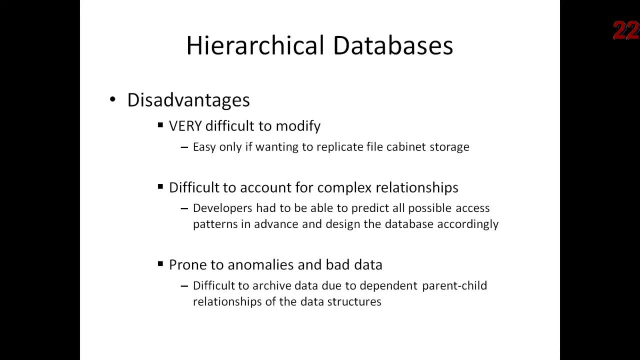 for complex business relationships. Also, we had in the small print here: the developers who built the application had to know how data was going to be accessed. That slowed down how quickly companies could modify their data. That was slow. They had to, so businesses. 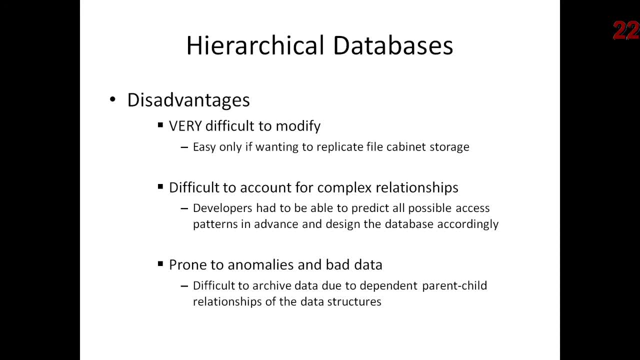 were not very flexible. The takeaway from this: businesses were not flexible, It took a long time still to process orders And not very nimble. Not very nimble, Prone to anomalies and bad data. I already mentioned a little bit how people would get sneaky. 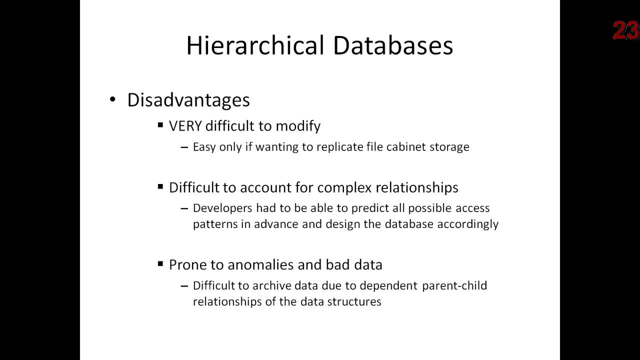 and put hidden copies of data that weren't widely shared. So it was possible to have inconsistent data records for similar entities like suppliers, customers, parts. All of a sudden there's two or three or four locations. Which one holds the most accurate data? If we are? 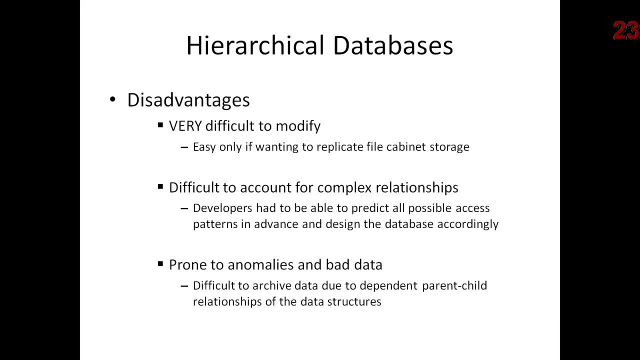 running reports on old locations, old data. we're going to be making decisions on old data. It's not going to put us in position to be very competitive, Unless, of course, our competitors are struggling with the same challenges. Complications over time. 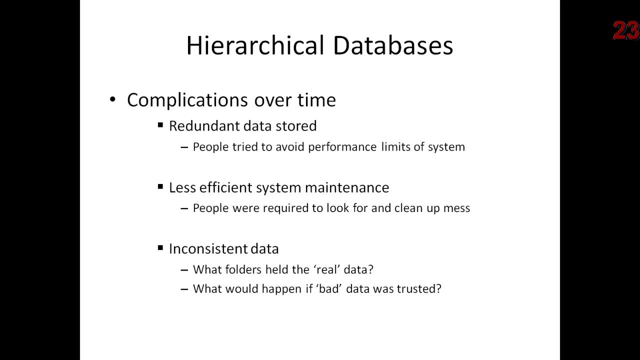 I mentioned again Redundant data. People tried to get sneaky, avoid performance limits, Less efficient system maintenance. Many people were required after people started getting sneaky. we then had to hire people to go clean up the sneakiness. 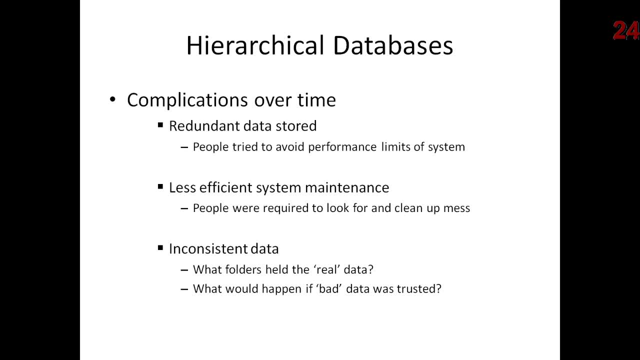 It's like, wow, Wouldn't it be nice just to do business, but we have such a high number of people required just to make sure things get processed correctly And then, when they don't get processed correctly, to go around and clean things up. 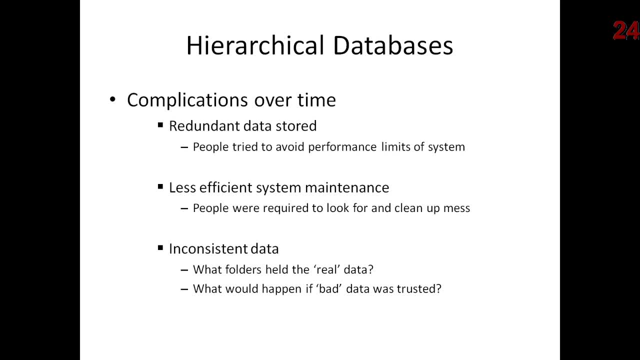 It's like having a bunch of janitors- Lousy analogy. We won't do that. Inconsistent data: What folders hold the real data? These are the complications that were faced over time with the hierarchical databases. Now we're only talking about a 15 to. 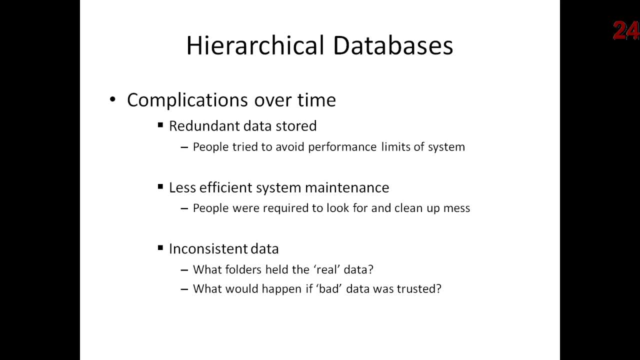 20 year window where this was experienced, Eh 25 years Post World War II to 1970, give or take 25 years and probably into the mid 70s. hierarchical systems were the dominant platform, Dominant way of leveraging database design. 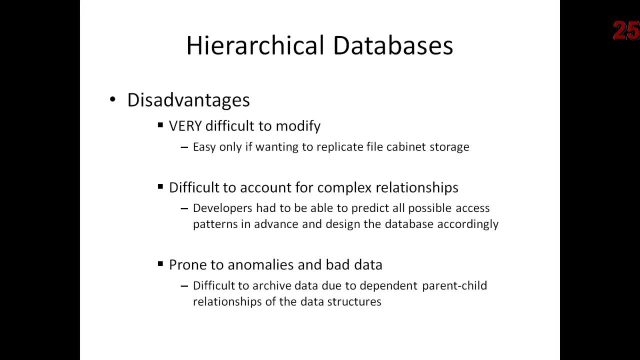 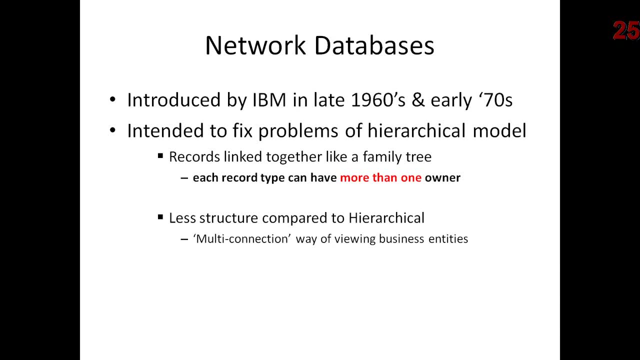 COBOL. If anyone knows that, Oop, I hit the up arrow, We're going down this direction. So that led to the network database design. There were complications with the hierarchical system, So it's like, well, what can we do to fix this? 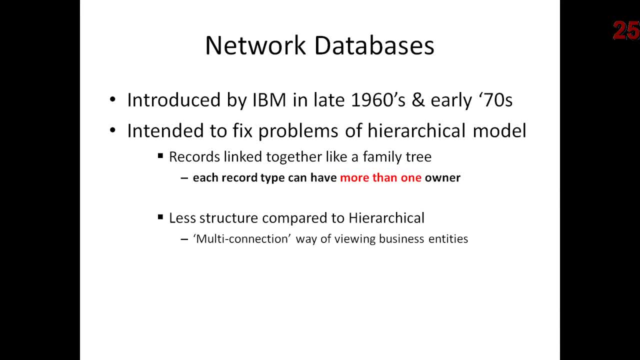 What were some of the easier gets to fix And it was solely intended to fix the hierarchical model. Well, if you remember, records had only one parent in the hierarchical system. Only one parent. The businesses were screaming, you know, we need to have multiple. 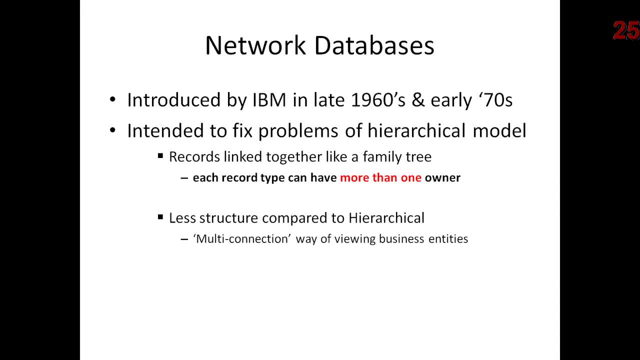 copies. We need to have multiple ways of correlating data to other data, For example employees and the locations they work. It's very difficult to vertically dive into each file just to see if there is a record that we are looking for in that location. 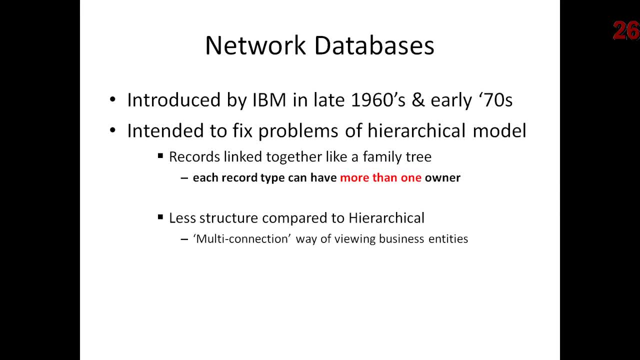 Imagine driving to a library just to see if they have a book And you have to go to the bookshelves. You can't look in a card catalog, Have to drive physically to a library and go through the stacks to see if a book is physically present. 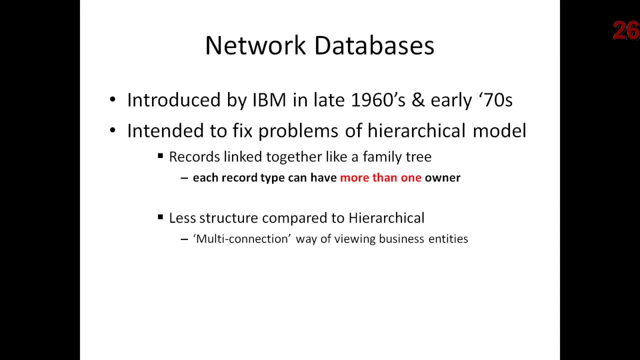 It's not there. Great, Get back in the car and go to the next library. Can't call ahead. Gotta drive Now. that's just going from one library to another. Imagine driving to five hours away. I'm being a little bit more dramatic, but imagine. 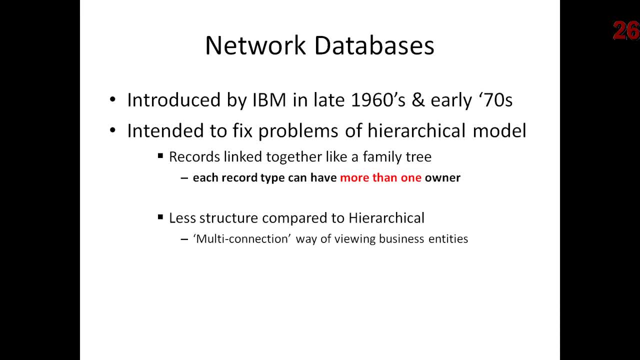 if you have to go to Portland from Seattle, which is about a three hour drive, and then we're skipping Tacoma on purpose, because who's kidding whom? Who wants to go to Tacoma to find a book? Just kidding. Then Spokane, which is a 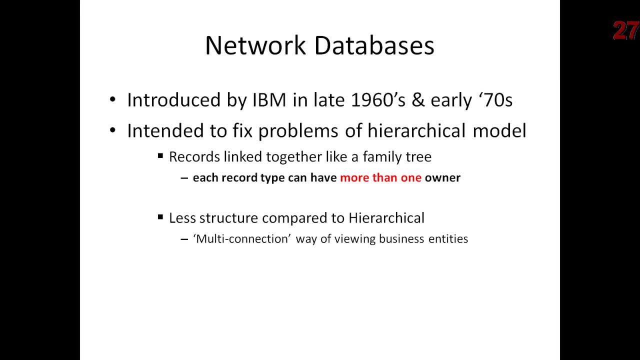 five hour drive, perhaps, from Portland. So the analogy is: it's very, very inefficient to scan for data, Inefficient enough that IBM, whom developed the hierarchical model, was like: yep, this is not scaling, This is not efficient. We have to have 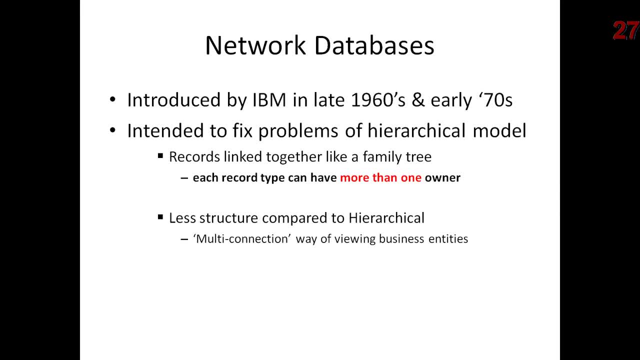 a different way. What did they do? They came up with a network model that allowed records to have multiple parents, multiple owners. That's the big takeaway: We don't have to know the exact details. This is less structure than the hierarchical model. 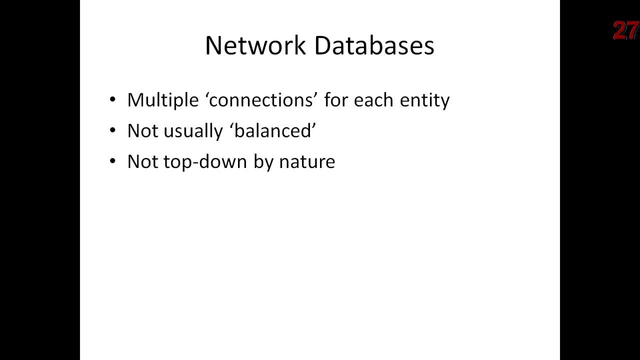 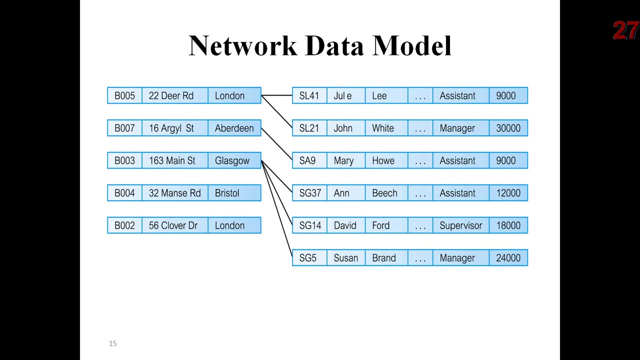 I put multi-connection, a way of viewing business entities. When we say not usually balanced, it's not top-down, We have multiple pointers. Let's use an example here. We can now search by the branch, for example, and we should be able to. 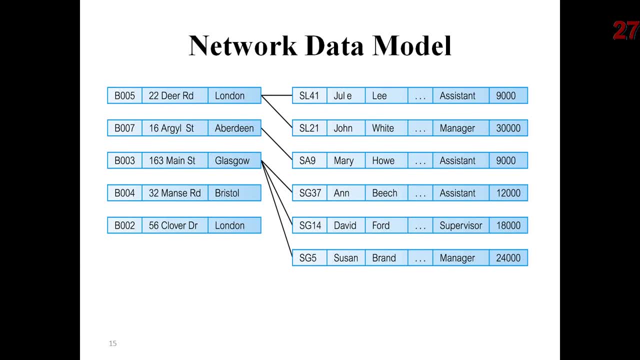 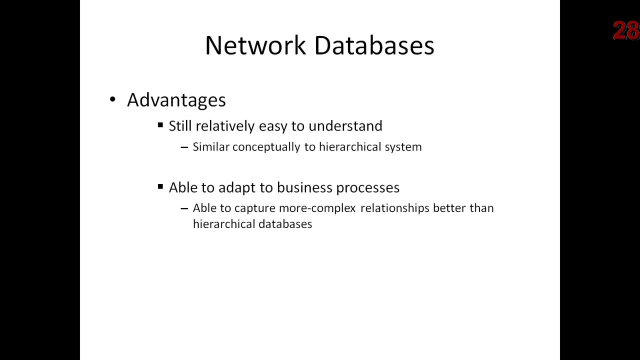 determine very quickly which employees work at which branch- A little bit more streamlined Advantages- still relatively easy to understand. It's still similar conceptually to the hierarchical model. We still have a similar way, a paper-based approach to the system. 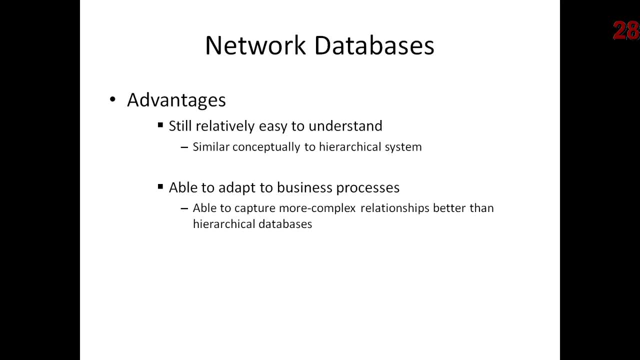 We're better able, however, to adapt business processes. We have a better way of aligning records to other records- Business objects- And this becomes more prevalent when we move to the relational data model, but we're still not. this is better than the hierarchical model, but it still. 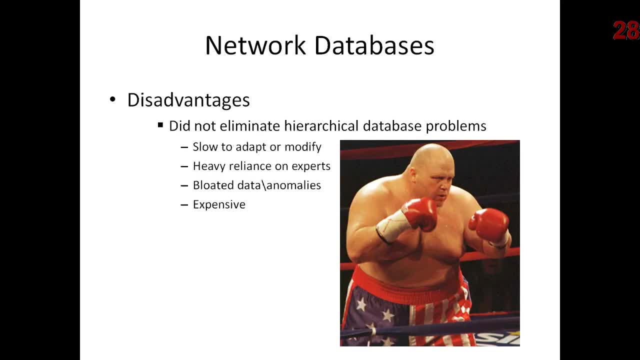 doesn't satisfy everything that business needs. This is not my dad Disadvantages. It did not eliminate most of the problems. We were still slow to adapt or modify applications. Heavy reliance on experts. We had bloated data and anomalies Again. 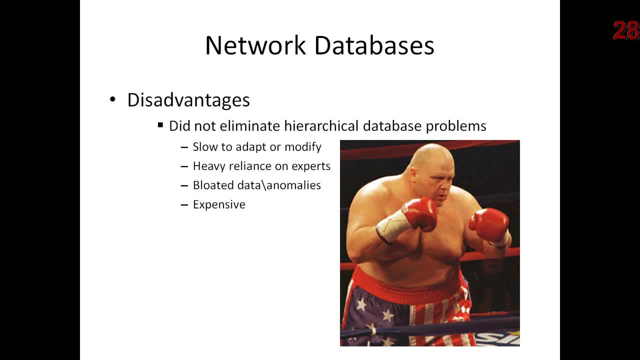 multiple copies of data being stored. If we were going to reference business locations, we would probably pack or stuff other relevant data like what employees work there, what products are sold at that location. It was kind of like a bank and I just converted it to like a warehouse. 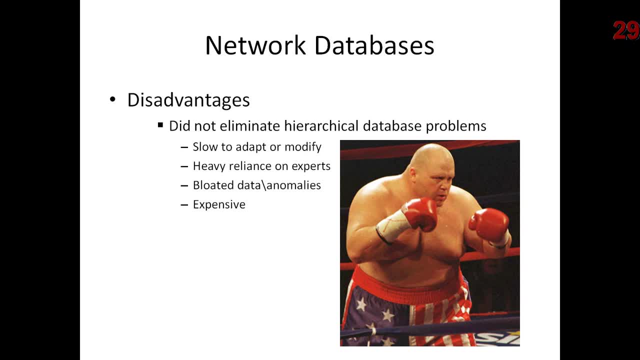 or a retail store. The idea is we're going to have those objects stored in multiple locations because we may be accessing the data for different reasons and we don't want to have to collect data on employees, then go out and collect data on branches and then go collect data. 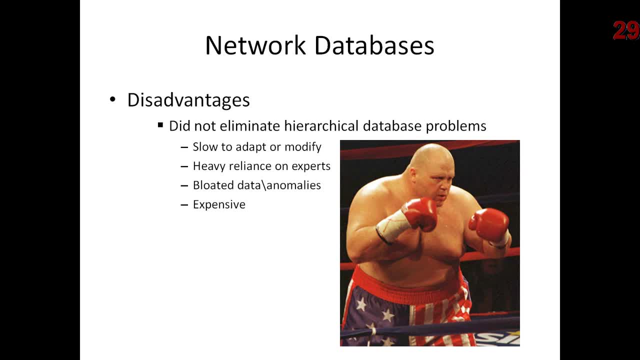 on products. We want to stuff all that data in there in each location, Because we don't know what questions we're trying to answer. Obviously, the problem is it takes longer to write the data when there is a transaction. It takes longer to fix. 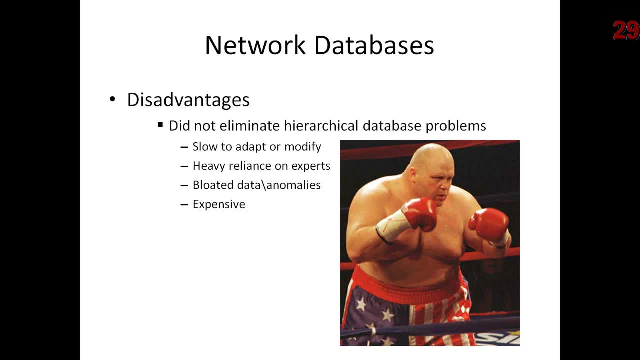 if there is a discrepancy between the data at different locations on disk, It becomes bloated and there's data anomalies, meaning there's inconsistency And again very expensive. We have more people that have to be staffed up. We have still expensive. 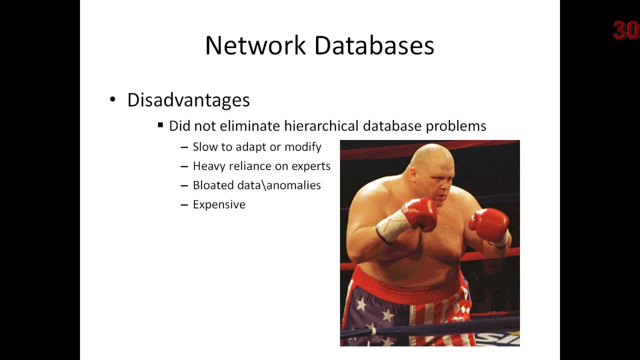 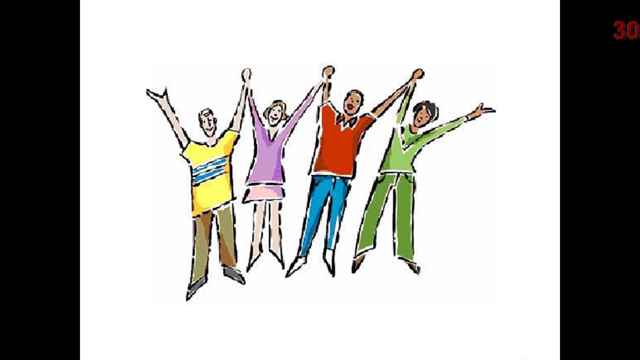 hardware. We have highly, highly trained people that are commanding large salaries, Very expensive. Still more disadvantages with the network database model. That is the high level overview of the hierarchical and network database systems. Thank you. 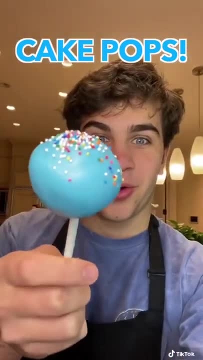 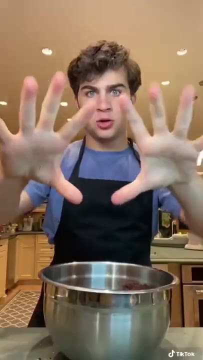 You need to know how to make cake pops. They are one of the easiest desserts to make and they're so delicious and pretty trendy. Take your favorite cake. I'm making it from scratch. You can use a box and just dump it into a bowl- Go crazy, Then you're going to have to get your. 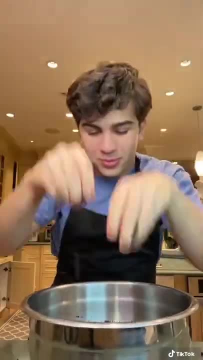 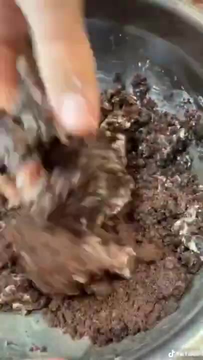 hands in there. Mash it up real good until you only have crumbs left. Then take your favorite frosting and just dump it into the cake. Mix it all together. There's no real measurements here. You just add enough frosting until you get this doughy consistency. Take a big chunk of cake and 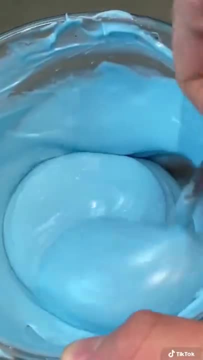 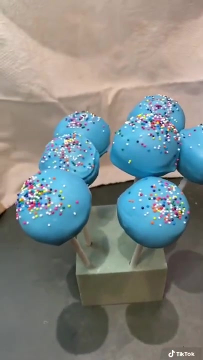 roll it into a ball, Freeze your cake balls and then melt some chocolate or candy melts, Dip a stick into the chocolate and then into a cake ball, Freeze again and then dip the cake into the chocolate- So satisfying. There you have beautiful cake pops. Check out my Instagram and